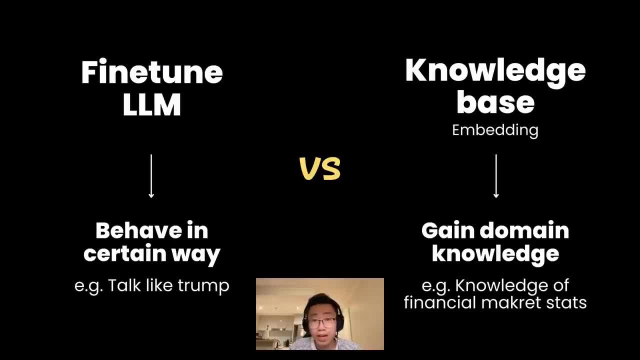 broadcast interview transcripts into large-language model so it can have a certain type of behavior. But if your use case is that I have a bunch of domain knowledge, like a legal case or financial market stats, fine-tuning is actually not going to work because it's not good at providing very accurate data. Instead, you should use fine-tuning. If you have a bunch of domain knowledge, like legal case or financial market stats, fine-tuning is actually not going to work because it's not good at providing very accurate data. Instead, you should use 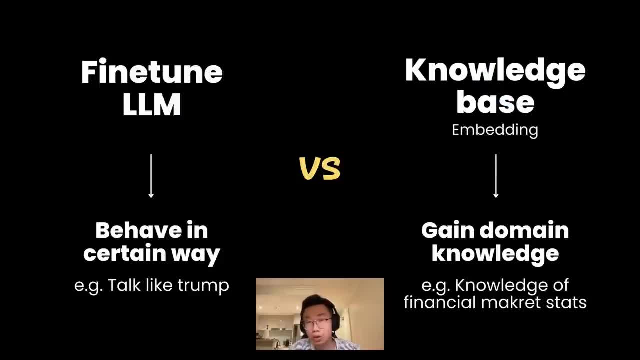 embedding to create a knowledge base so that when someone asking which stock has the hightest price movement easily, it will gather real data and feed it as part of the prompt. So those two methods are two different use case. A lot of time you can just create embedding, But fine-tuning is still super. 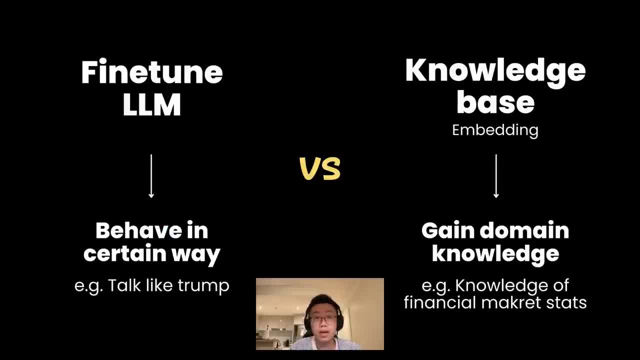 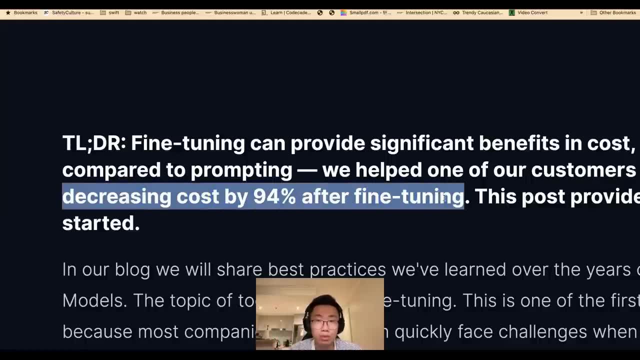 valuable for you to create a large-language model that have certain behavior. It's a pretty way to decrease cost because instead of adding a big chunk of prompt to making sure large-language model can behave in a certain way, you can just teach large-language model, so you cut the cost. 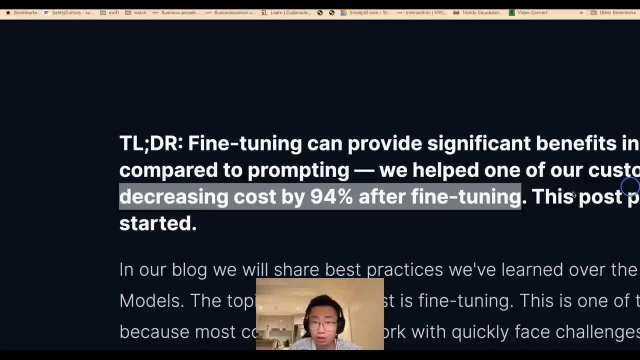 So there's still a lot that you want to learn from this example And, if you want to learn more, another legit use case where you should fine-tune the large energy model, And that's I want to show you a step-by-step case study. 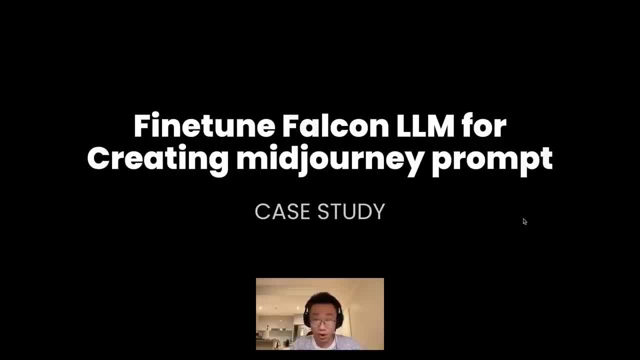 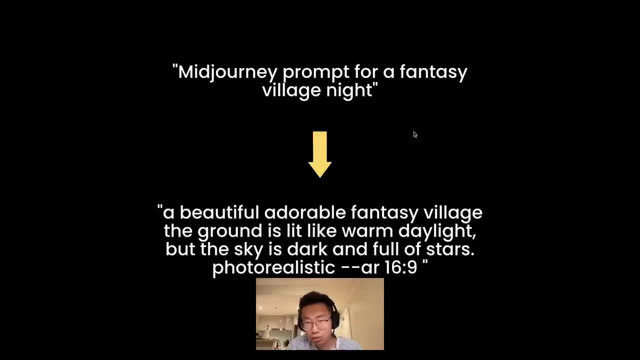 How can you fine-tune a large energy model for creating mid-journey prompt? And this is a great use case because it is not a task that base model like GPT are good at. What I want is a large energy model can take a simple instruct like this and 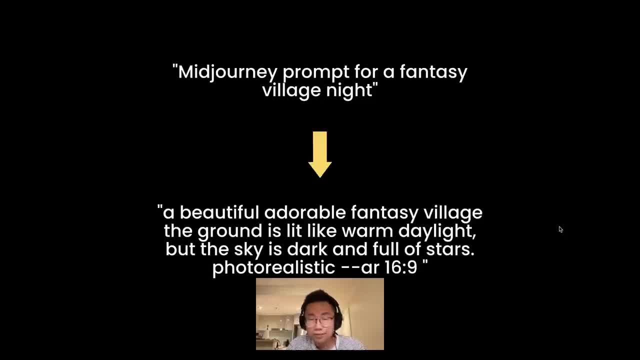 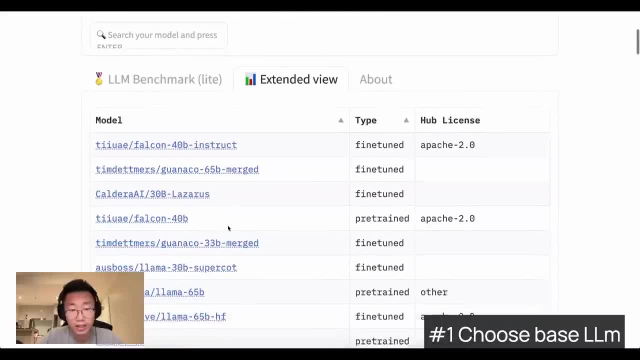 turn it into a mid-journey prompt. So let's get started. Firstly, we need to choose which model to use for fine-tuning. HuggingFace has this leaderboard for all the open large energy model And you can take a look to choose the one that suits you most. 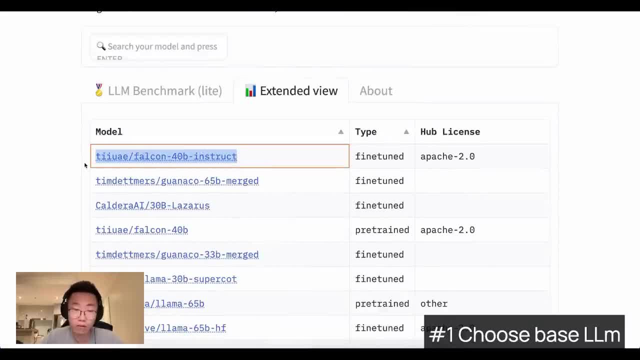 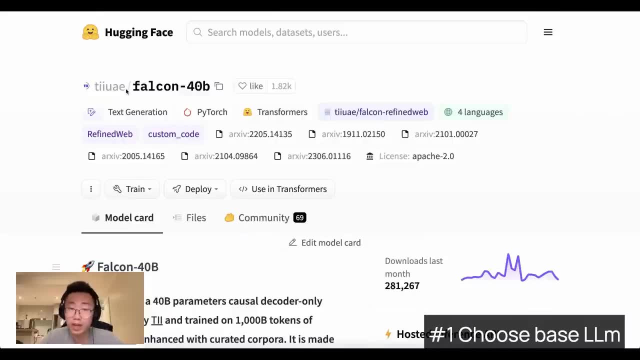 The one I'm going to use is the Falcon. It is one of the most powerful large energy model that has been our number one place on the leaderboard in a very, very short time, And it's also a few ones that are available for the commercial use. 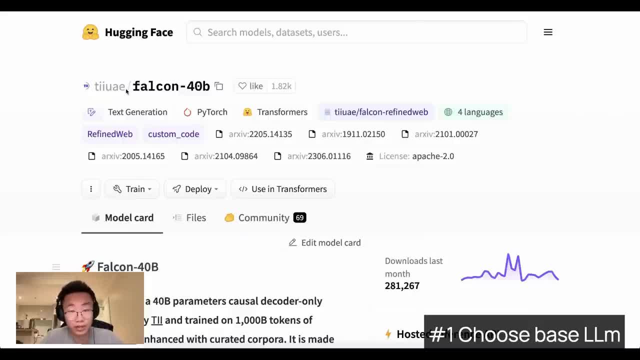 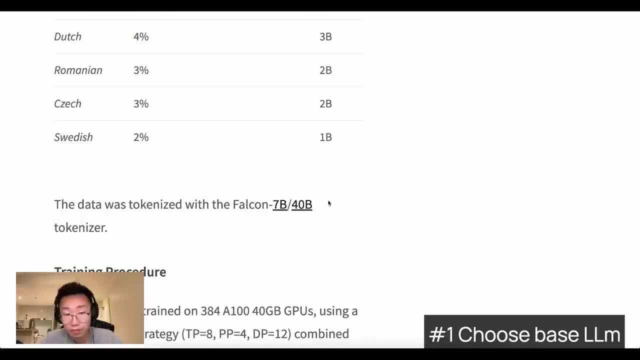 So you can actually use this for production level products for your own company, And it's a chain not just on English but a large set of different types of languages like German, Spanish, French, And it has a couple of versions- 40B version, which is most. 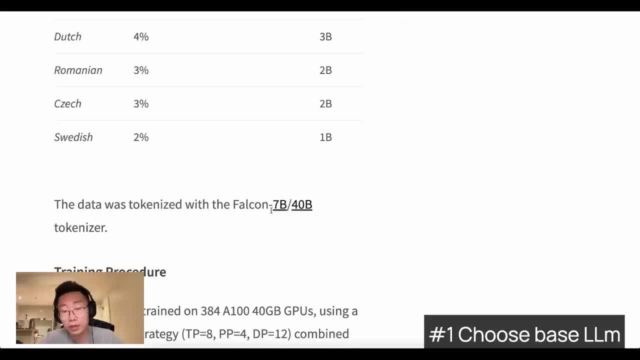 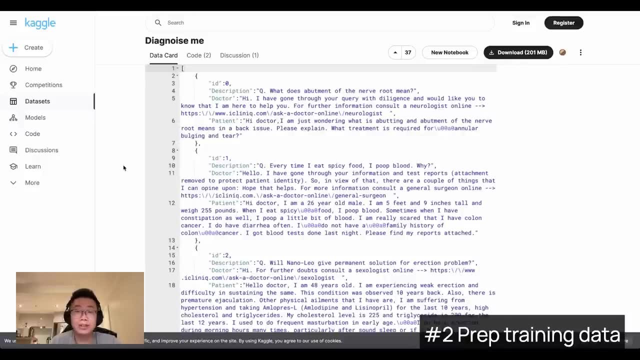 powerful, But also a bit slower. think about more like GPT-4,, but it also has 7B version, which is much faster and cheaper to train as well. The next, which is most important step is getting your data sets ready. 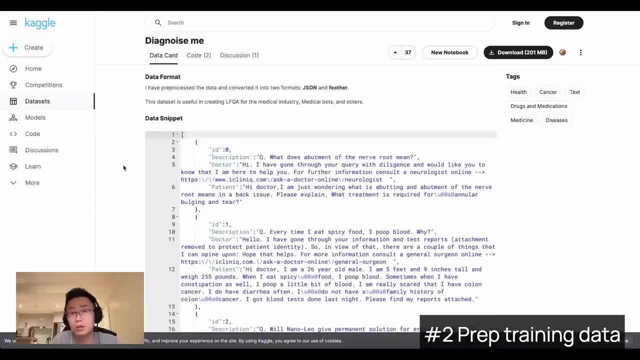 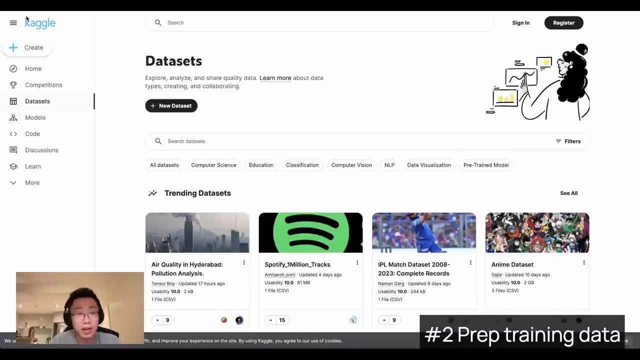 The quality of your data set decides the quality of your fine-tuning model. There are two types of data sets you might use. One is public data sets that you can get from internet and their model place. You can get it like Kaggle, which is a data set library that has a wide 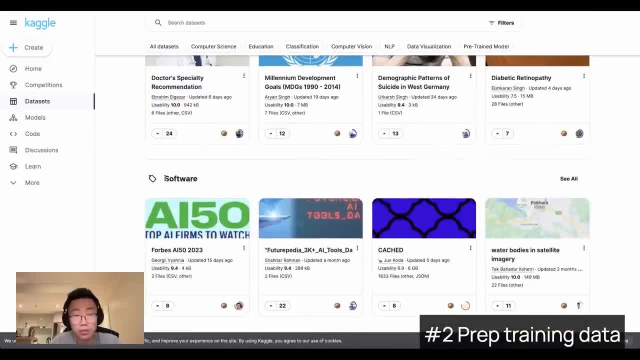 range of data across different topics, like sports health software, And you can just click on any of them Preview The details of the data And, if it's good, you can download to use. On the other side, Hugging Face, also have very big data set library. 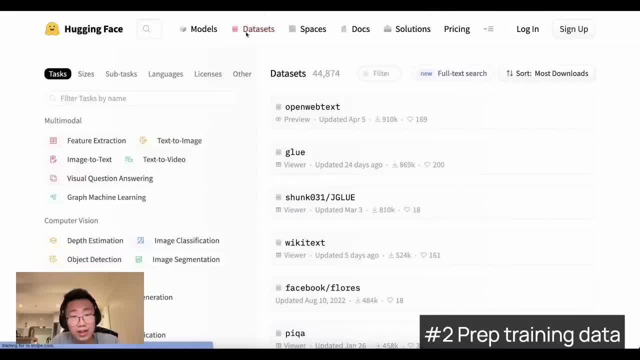 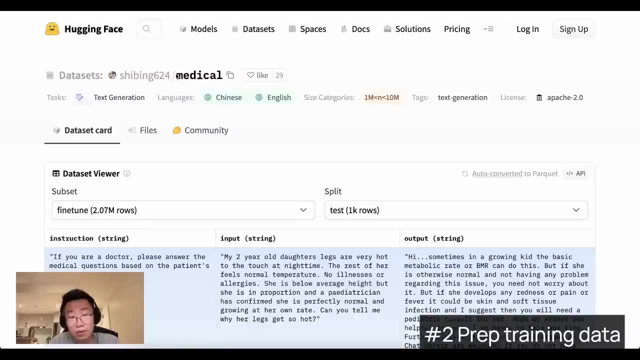 And to find the ones that you will use for training. large language model. you can click on data sets, move down here, try to find the text generation and you can try to find the relevant data sets that you want. For example, this is one public data set for medical related Q and A data sets. 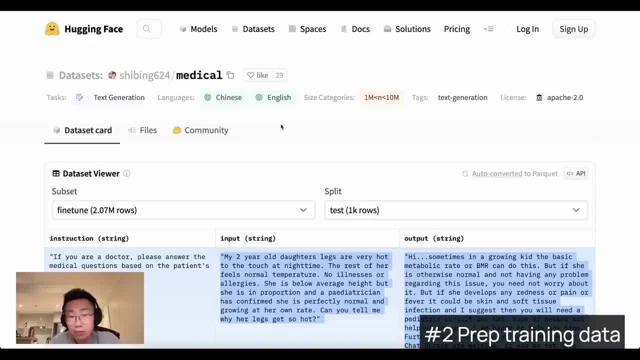 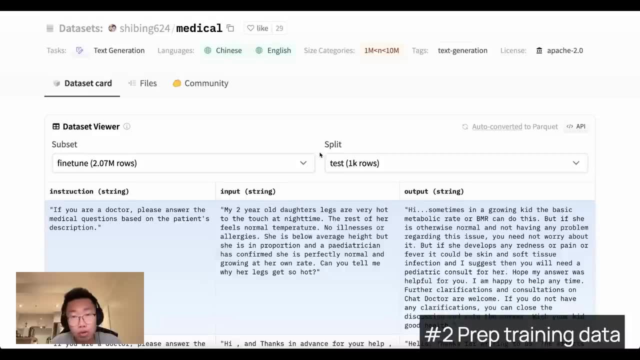 You can preview what data actually inside. but on the other side, I think the most of the use case for fine tuning is actually use your own private data sets That is not available anywhere else. It actually didn't require too big a data sets. 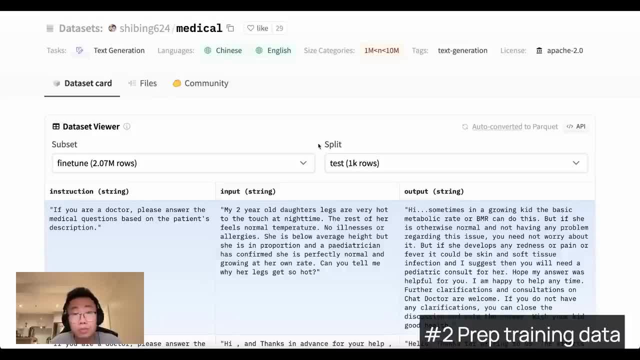 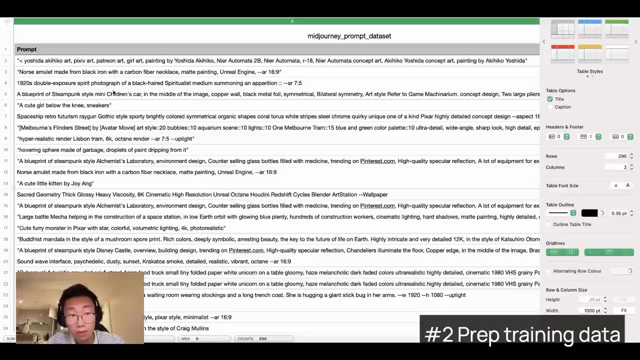 You can even start as little as a hundred rows of data, So it should be still manageable. So this one tip I want to share is that you can actually use GPT to create a huge amount of training data. For example, I have collected a list of really high quality mid journey prompts. 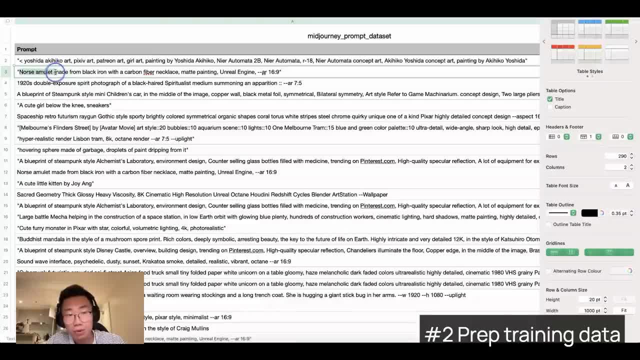 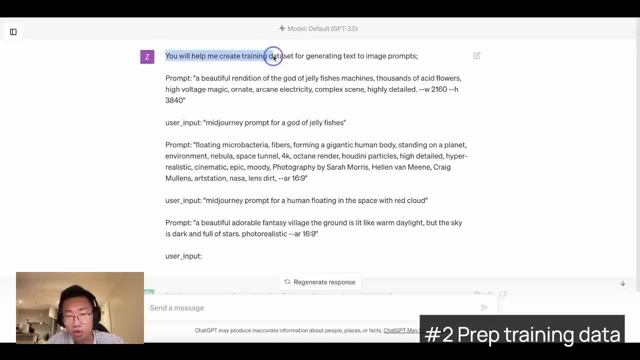 and I want ChatGPT to reverse engineer, generate a simple user instruct that might generate this mid journey prompt, And what I would do is give ChatGPT a prompt like this. you will help me create training data sets for generating text to image prompts. 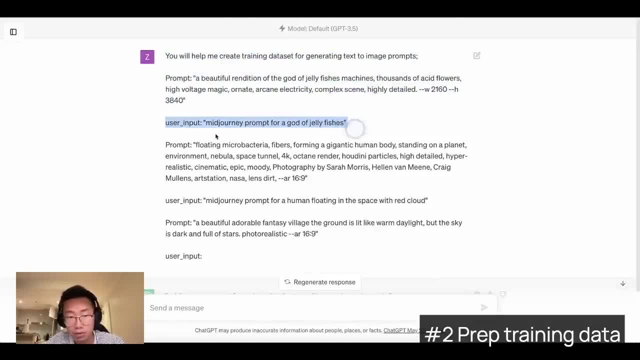 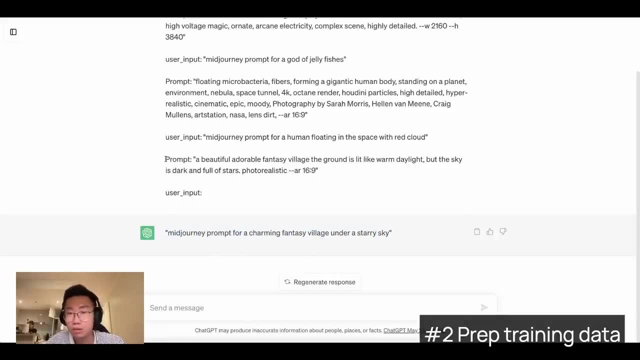 And then I'll give it a few examples. like this is a prompt and this is a user input And in the end it will start generating a user input that pair with this prompt which I can use them as a training data for fine tuning Falcon model. 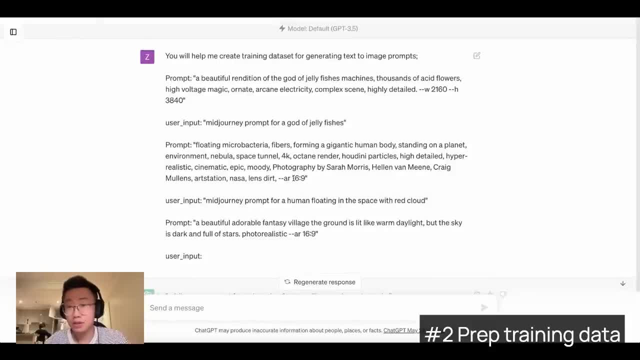 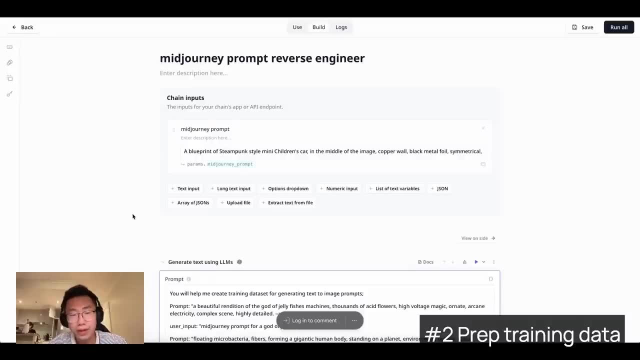 And all we need to do just repeat this process for hundreds or thousands of rows. But luckily there are platforms like relevance AI, where you can run the GPT prompt at scale in bulk. For example, I can create an AI chain with this input variable called mid journey. 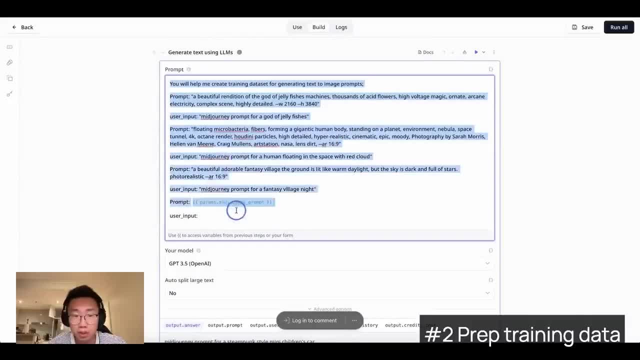 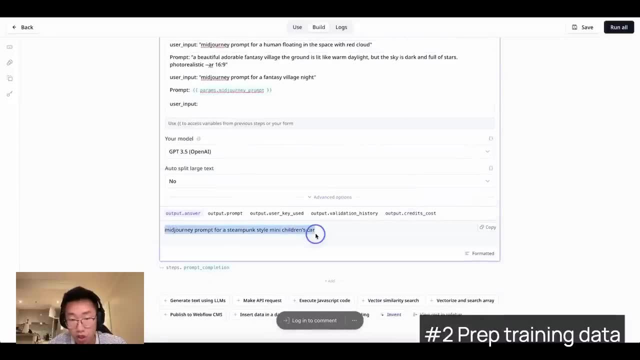 prompt, And then I will copy paste a prompt That I was using in ChatGPT, but point the last prompt to the variable that we created here and let's run this So you can see it is working properly, as it generates a user input. 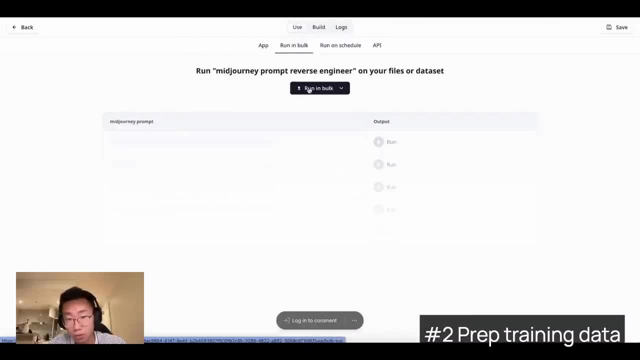 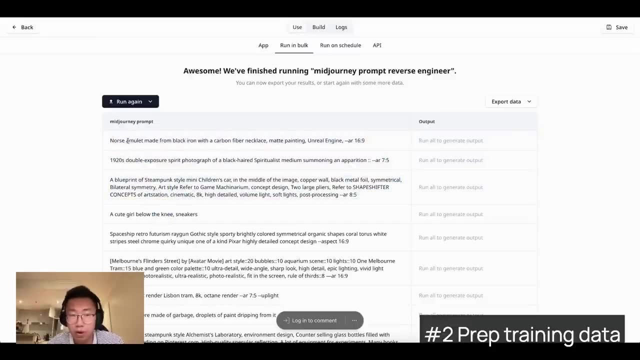 And all we need to do next is go to the use tab, This run in bulk option. allow me to upload the whole CSV file of the mid journey prompt, and then it will import the whole CSV file and run the GPT prompt for every. 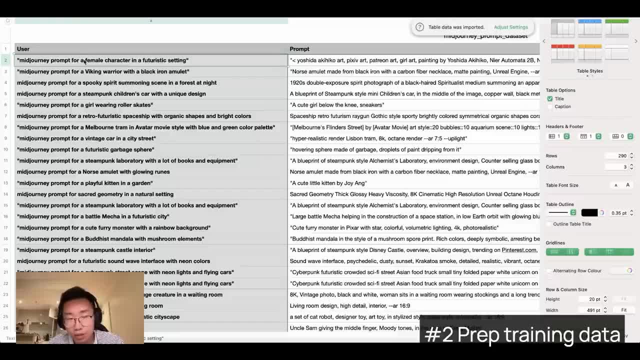 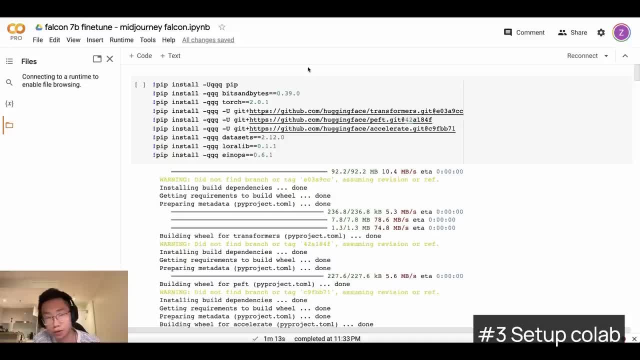 single row hundreds of times automatically. In the end, I can have the training data like this. So there's a pair of the user input as well as a corresponding mid journey prompt. So now let's fine tune the Falcon model. I'm using Google collab as a platform to fine tune the model. 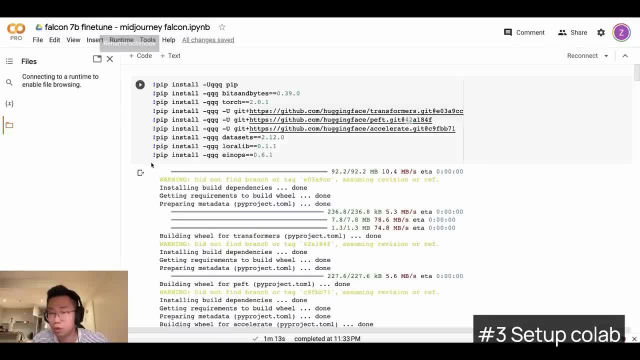 And I decided to use a seven B version, which is much faster. but if you want to use for 40 B version, it's basically the same code. You just need to find more powerful computer. before you run this, making sure you check the runtime type and choose a GPU, and at default I think you will be. 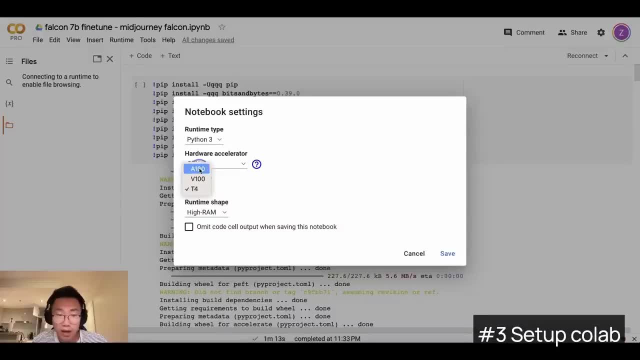 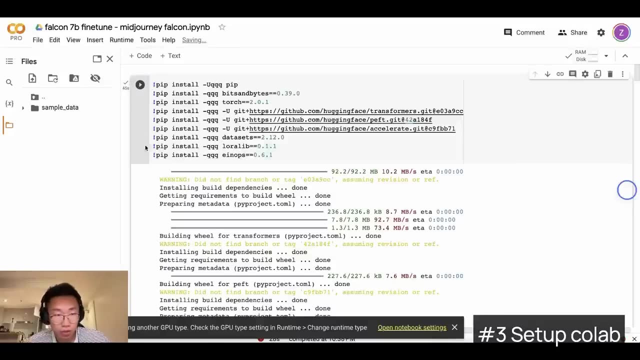 on T4 version, which still works, but I have upgraded so I can choose a hundred model, which will be faster. So first let's install a few libraries. Once it's finished, you will see a little check mark here Then. 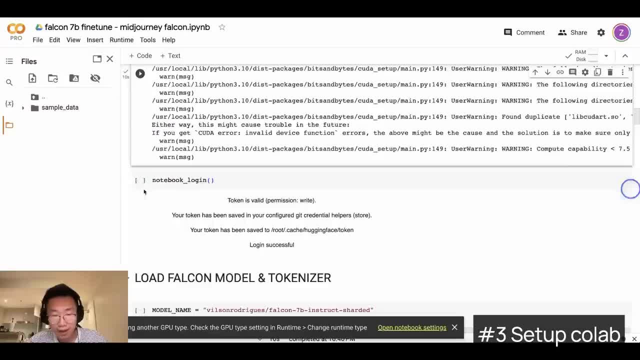 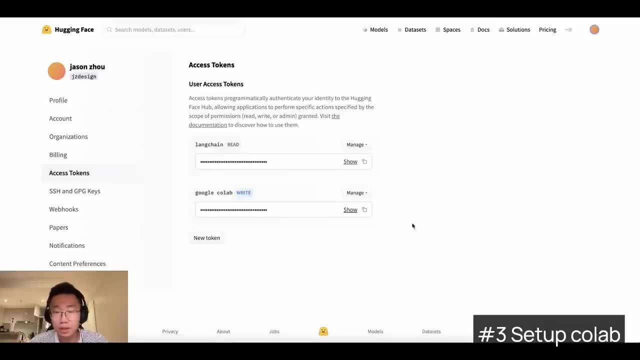 Next step is we will import all those libraries- Okay, great. And you will run this notebook login, which will ask for your hugging face API key. If you don't have hugging face account, just create an account and then copy the. 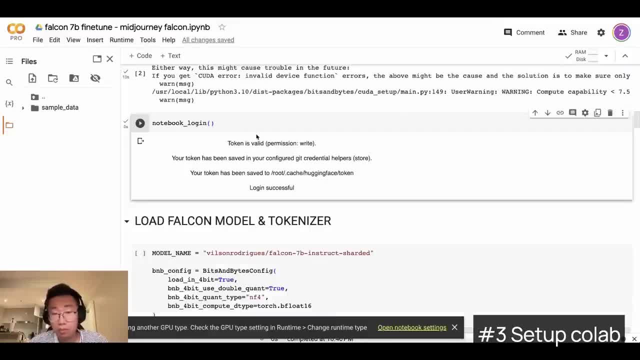 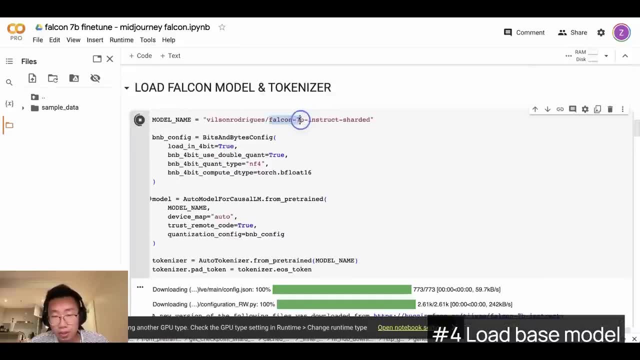 link here and paste here. We will need to use hugging face as a way to upload and share our model, And next thing we will do is we will try to load the Falcon model and tokenize it. first, And here's the model I choose is seven B: instruct, share it. 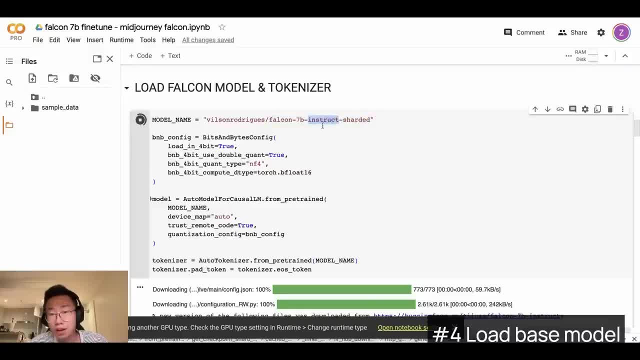 So instruct is a fine tune. seven B model specifically for conversation. So think about it. Let's chat GPT versus GPT three and share it. Just a version of 70 model. and share and share is this version of seven B model. that will be faster and easier to run. 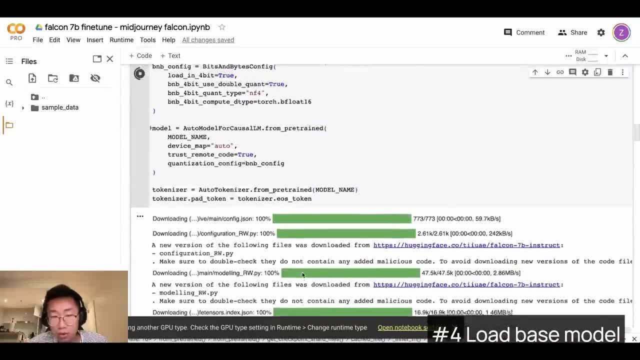 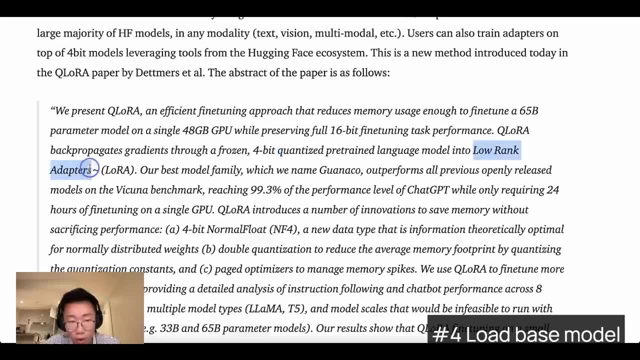 And it will take a while for you, And it is downloading the whole models. It will take a while. Okay, So the model is downloaded and then let's load the model Q Laura is a specific type of method called low ranks adapters, which is one way to. 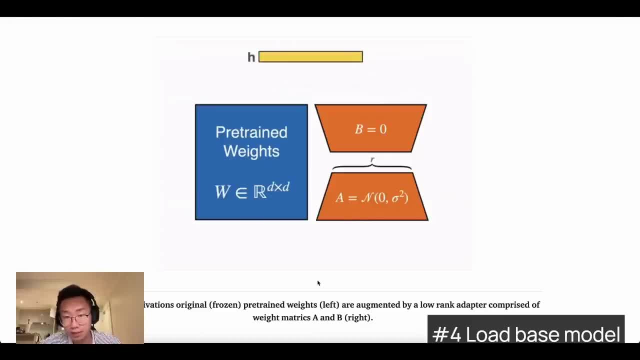 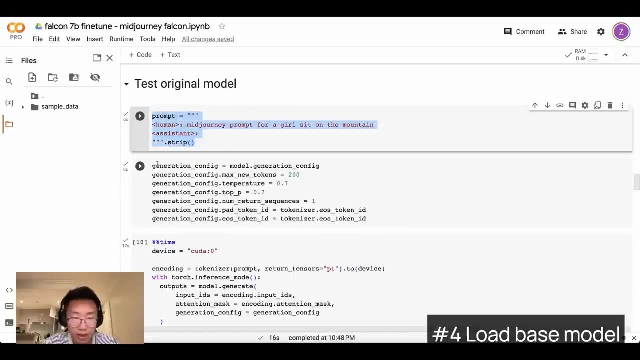 find you in the large language model much more efficient and fast before we find you in seven B. let's try this Prompt with a base model to see what kind of results we get. So I will create a prompt and then start loading a bunch of configuration for the model and 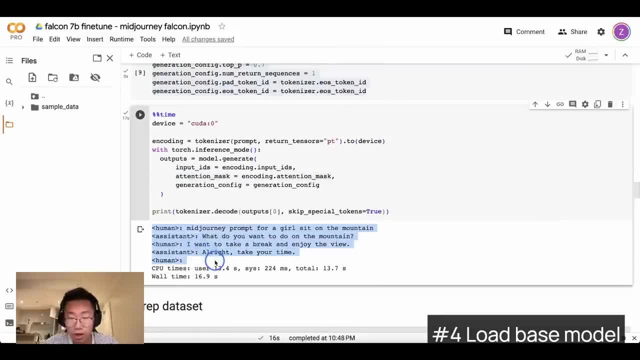 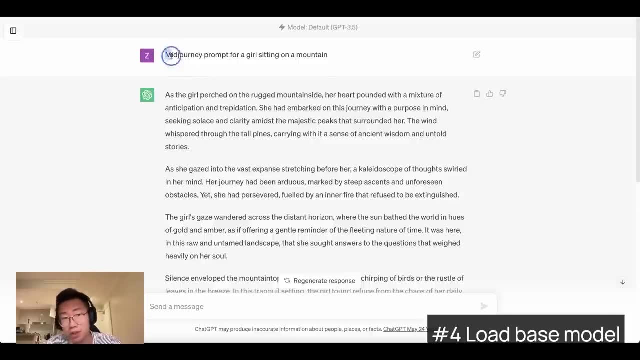 click around. So this is the results we get. It's not even close to generate a good mid journey prompt, as it didn't really understand the context And, as I mentioned before, even chat GPT is not doing a good job for this task. 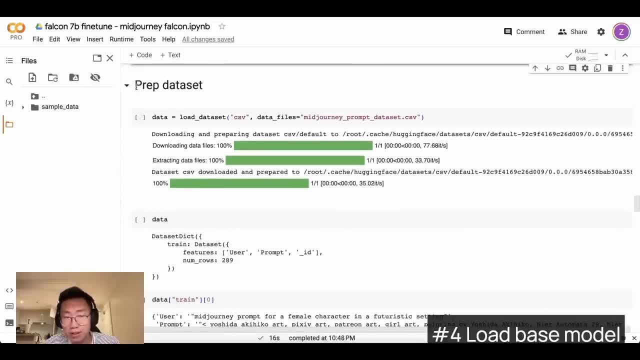 So I'm pretty curious to see the results, and let's first try to prepare the data sets. So what I would do is I would drag and drop the training data sets here And, once it's finished, I should See this file showing up on the left side. 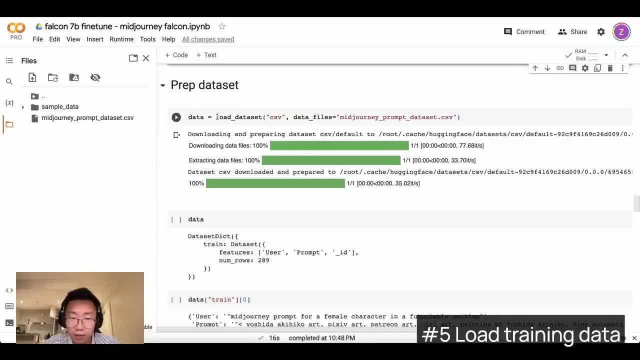 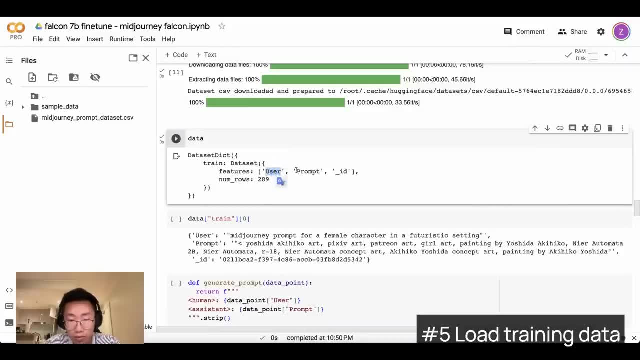 You can click on this file button to open this side panel, by the way. And then the first thing is: we will know this data set that we store locally and we can have preview of this data. So it has two column, user and prop. 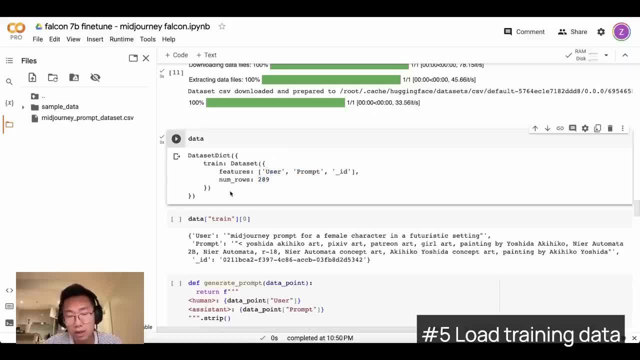 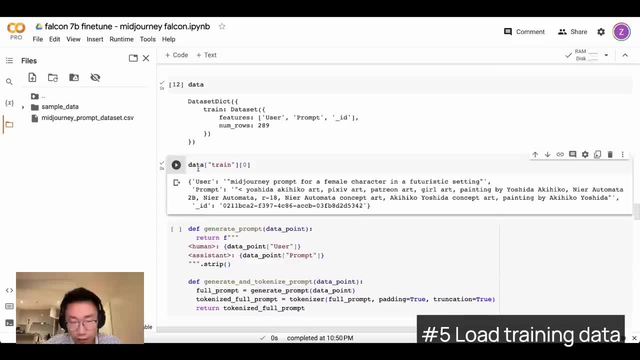 It has 289 rows. So this is actually another point I want to mention. You actually don't need a huge data set. Even a hundred or 200 rows can already generate a really good results for fine tuning, And if we pick up the first row, I can see the data. that is properly loaded. 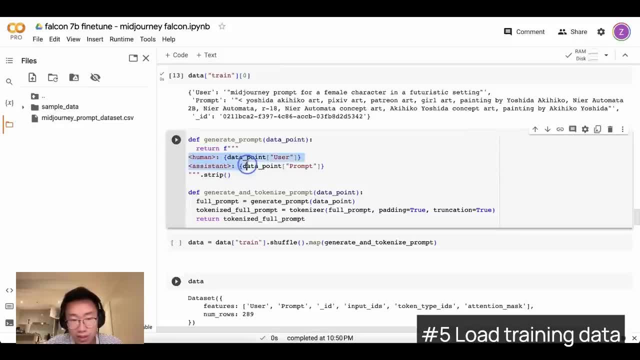 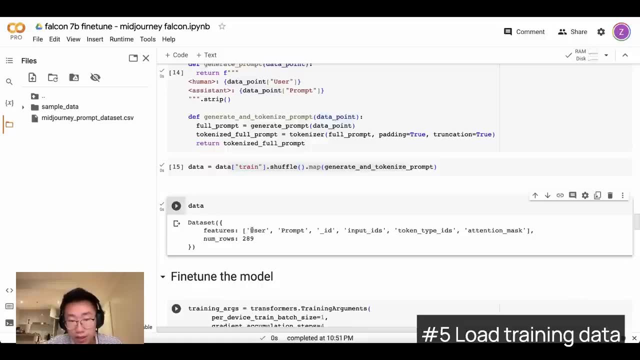 And then what do we want to do is to map the whole data Sets in this format- human and assistant- and then took a nicer prompt into our data set. So once it's finished, you can see the data set is fully prepared with input IDs, token type IDs and attention masks. 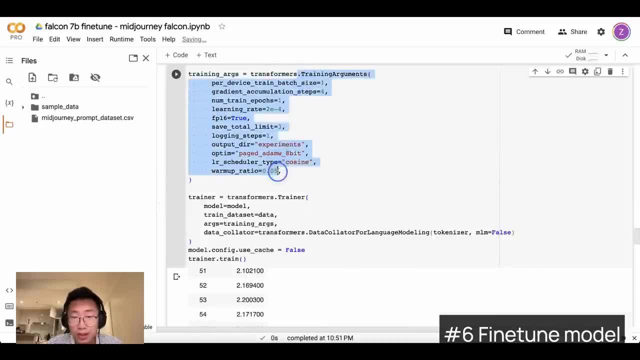 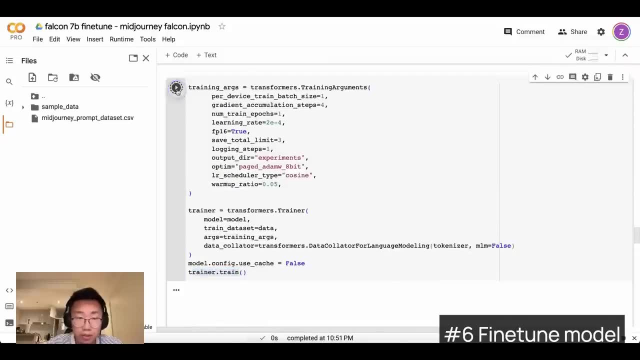 And firstly, we will need to create the list of training arguments, And you can use this one I have here as default, And then we'll just run trainer dot train to start the training process. And this will take a while for the higher end GPU. 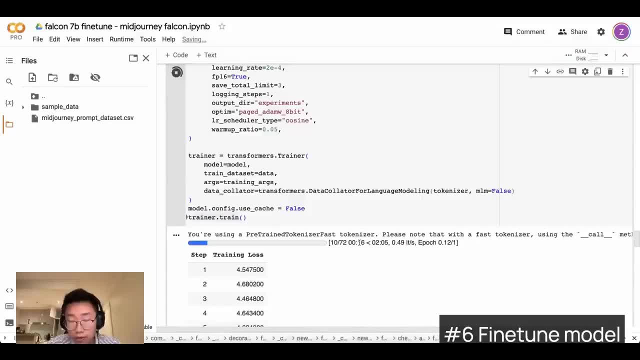 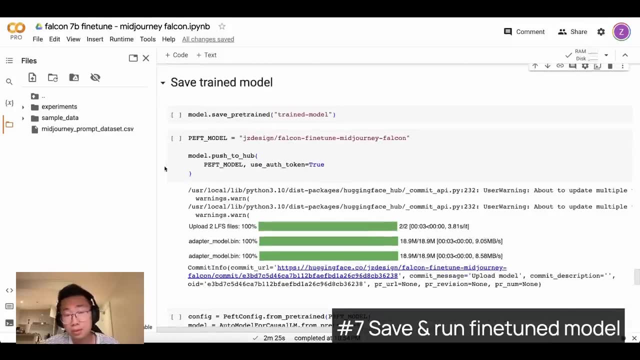 I choose. it take me two minutes. I think if you're using T four version, it will take you about two minutes. It will probably take you around 10 minutes. Okay, great, So we just finished fine tuning the model. The next we will need to save the model that we just trained. 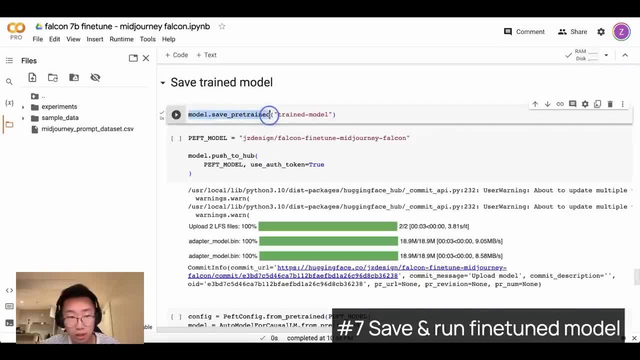 You can either save locally by doing model dot, save pre-trained, And once it is finished, you will see on the left side there's a folder called train model And inside this is model that we just created. but you can also upload this model to Hugging Face. 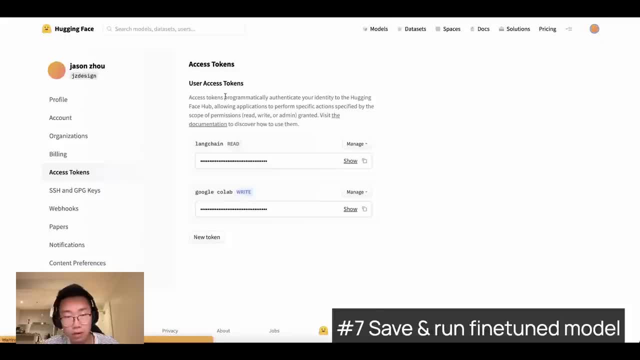 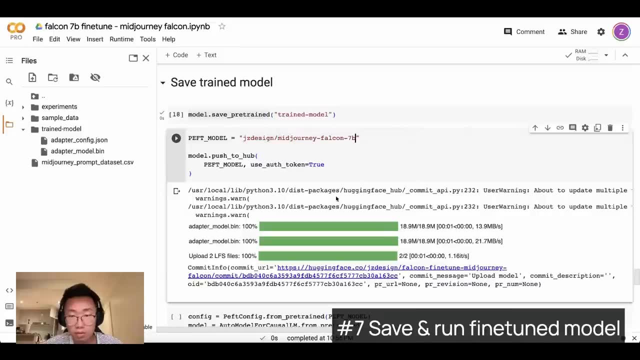 So you will come to Hugging Face. click on this new model under your profile. give a name and choose a license. Then click create model. Once you're finished, Then you can copy this and then coming back to paste on here. This will upload the model to your Hugging Face report. 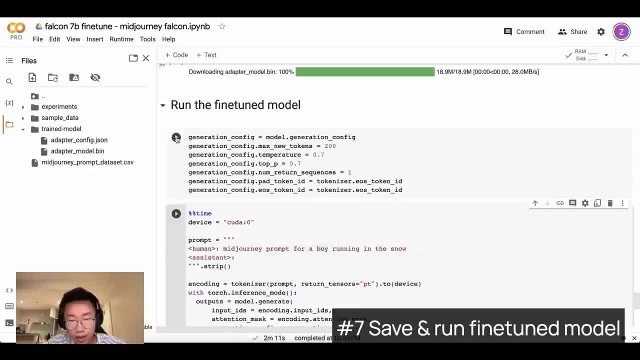 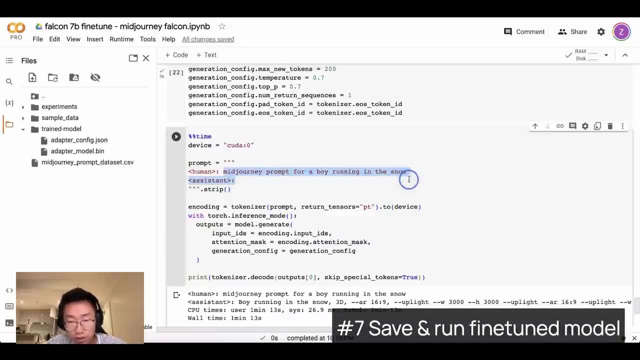 Okay, We successfully load the model and let's run this again. I will create a list of configuration for the model. Then I will create this prompt: mid journey prompt for a boy running in the snow and let's run this, Okay, great. 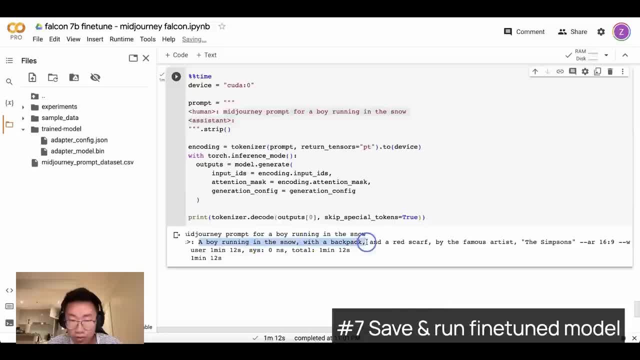 So we got this result. As you can see, it produced a really great prompt that I just tell you- that a boy running in the snow- and it is able to generate prompt A boy running in the snow. This is not a big deal.